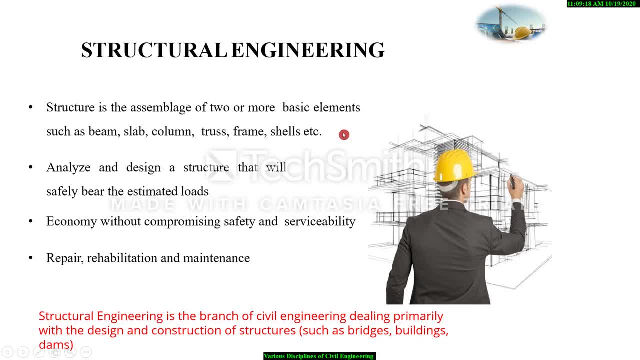 So before we start what is structural engineering, we should know what is structure. So structure is an assemblage of two or more basic elements. So structure is an assemblage of two or more basic elements, Such as beam, slab, column, truss, frame and shell. 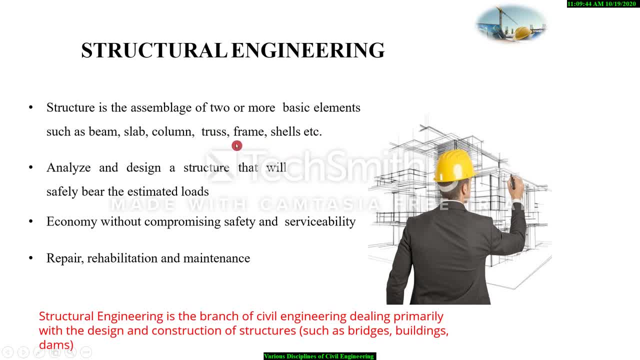 Such as beam slab column, truss frame and shell, So basically its assemblage of many basic elements- You have already heard of beam slab column- to form a main single member. Structural engineering is a branch of civil engineering. 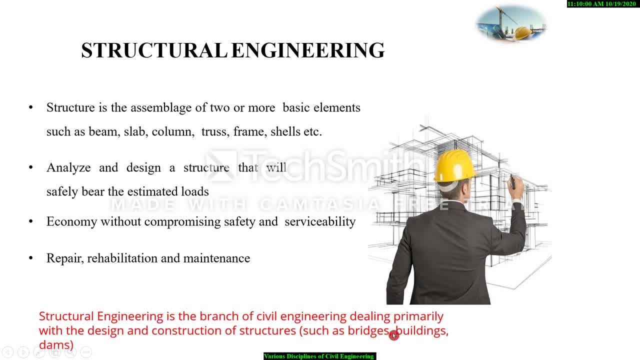 Structural engineering is a branch of civil engineering Which dealing with the structural engineering, with primarily the design and construction of structures such as bridges, buildings, dams. these are the main constructions and also there are small other constructions. a structural engineer should analyze and design the structure. so this is a figure showing the various assemblage of 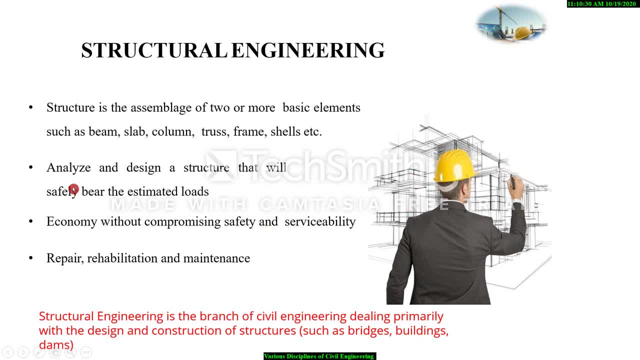 beams, columns, slats to make a building. so, similarly, the structural engineer should analyze the loads acting on the building or any structure and to design the structure to take the load, the estimated loads. we should also focus on the economy, without compromising on the safety and the serviceability. so the structure should be. 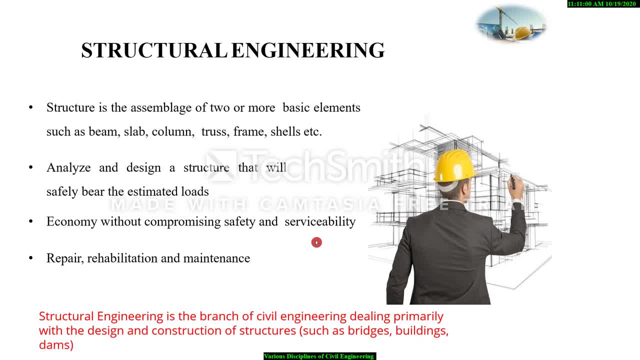 well as it should. serviceable, that means it should satisfy the functions on which we are building the structure. he is also interested in repairing, rehabilitation and the maintenance of the existing structures. so how to strengthen a structure is already weak due to the because maybe it may be considered long years ago, so it's all about repairing and 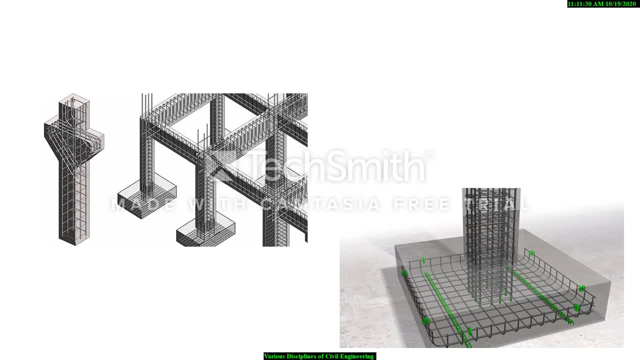 maintenance. so these two figures just shows the various structural elements. you can see a column, the rcc column, because there is reinforced steel reinforcement inside the concrete to give strength to the column. and also in the next figure you can see a combination of 14 foundation with reinforcement, the column with reinforcement and the. 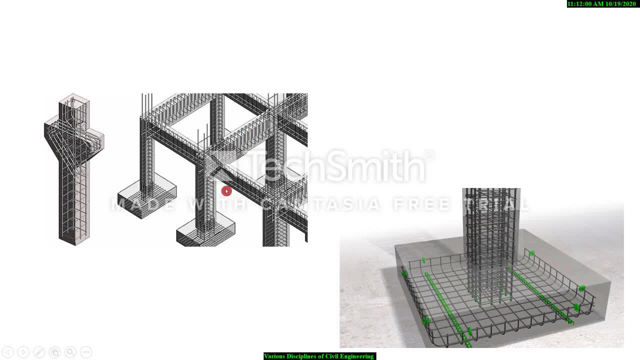 grid of beams with the reinforcement and how it is connected. so you don't want to study detail now, but just see and just know that there are reinforcement in the every reinforced human concrete frames and other structures. this in detail, the reinforcement for f14 as well as for the column. 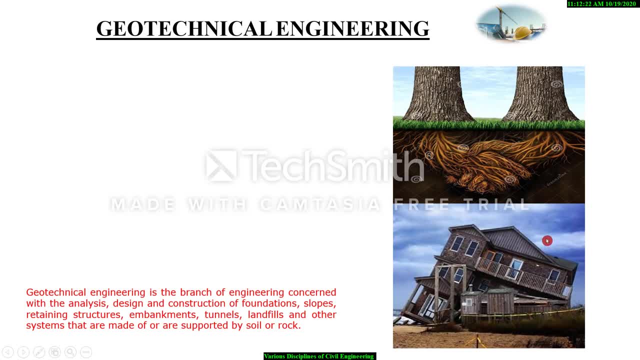 the other important discipline of civil engineering is the geotechnical engineer. so, as you know, civil engineering is a geotechnical engineer. so, as you, As we all know, every structure or every building which is made by a civil engineer is founded on the earth or the ground. 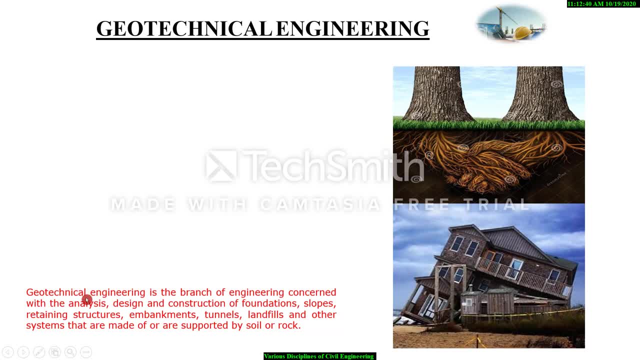 So the civil engineering. in civil engineering, the geotechnical engineering is a branch of engineering concerned with the analysis, design and construction of foundations, slopes, retaining structures, embankments, tunnels, landfills and other systems that are made of ore are. 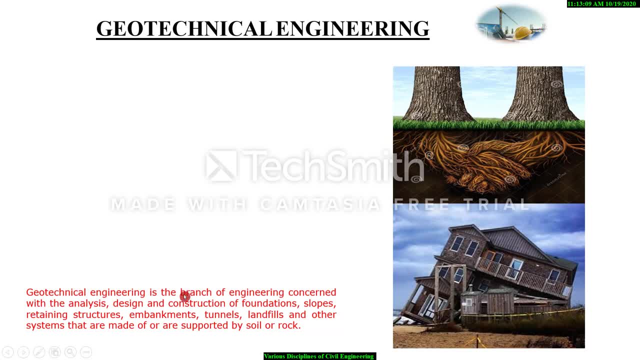 supported by the soil or rock. So anything which is done on the soil for engineering purpose, or even on the rock, comes under the geotechnical engineering. So you can see the figure showing a tree which is well rooted. So this root is very important. 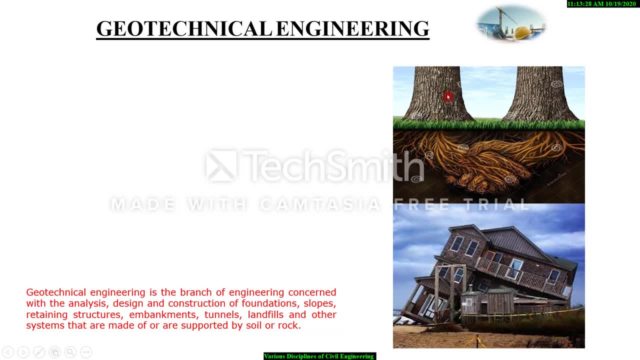 This root is very important. Well, rooting is very important for the stability and the growth of this tree. So you can idealize that this root is like a foundation and this is the building or superstructure. Similarly, in the figure, this figure shows the importance of the foundation and in adequate 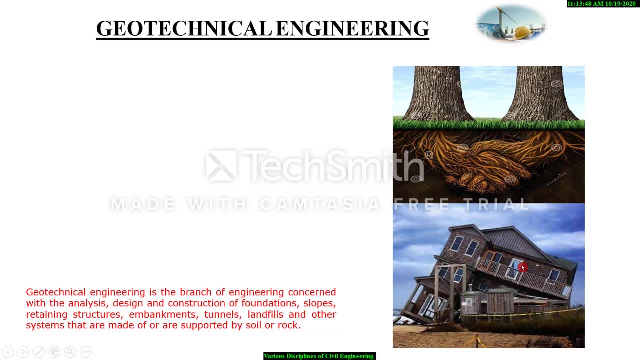 design or only design foundation may result in the total failure of the building. So a geotechnical engineer should We know to investigate the soil, to know the properties, basically the engineering properties of strength and other parameters, and the bearing means how much load the soil can take. 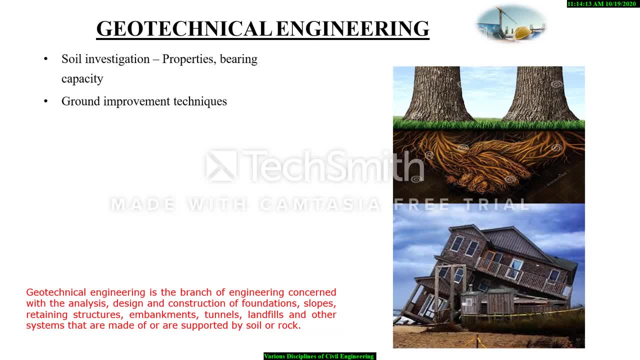 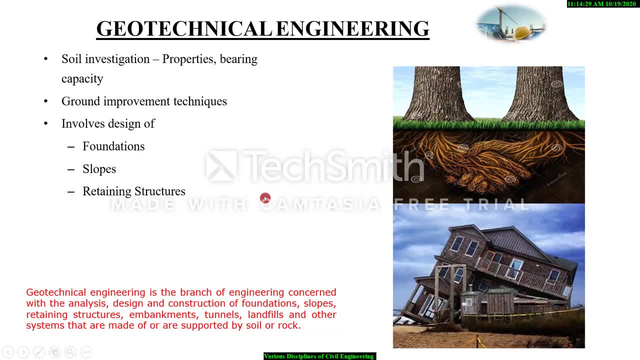 It involves the design ofators. It involves the design of properly heat retention structure. It involves the design of the acoustic we have seen in the structure of the foundation. It involved the large Mira Cascade. It was used for the whole construction. There are now one large floor, very large basement, medium, a large ground space area. 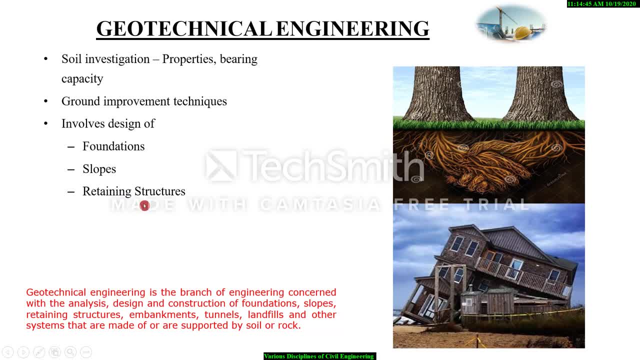 where the structure will emerge. The concrete structure is to be reaching more down over a single level that will make a replenishment structure, While in this structure you need reinforced from what is called a wetland base design below the road and also on the embankments and the earth dams. 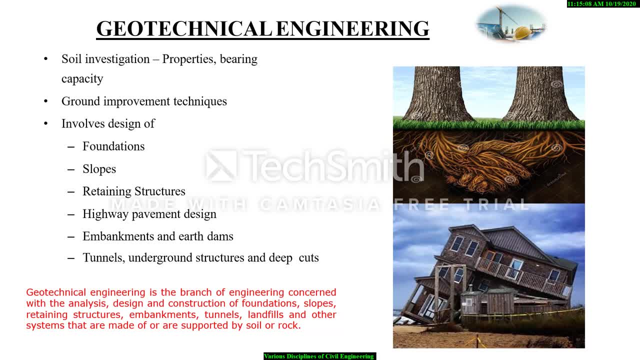 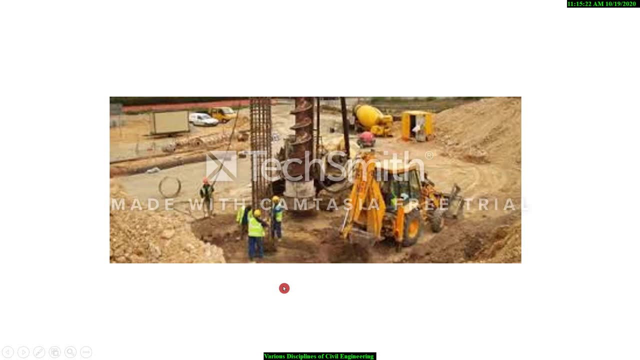 similarly tunnels like kudran tunnel and so other tunnels, which has to be drilled through rock or through the ground and also on the underground structures and the deep cuts. so this figure shows an side figure showing the installation of pile. the foundation can see a rigger that means this is used to drill the hole in. 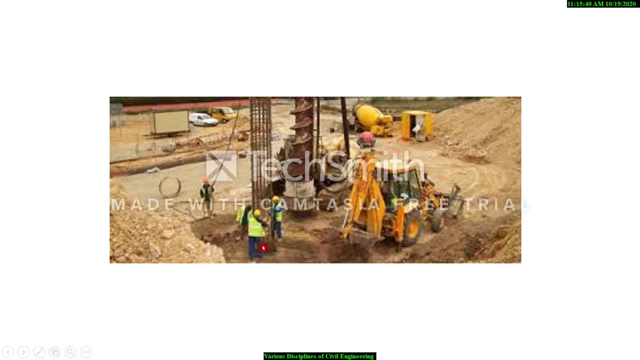 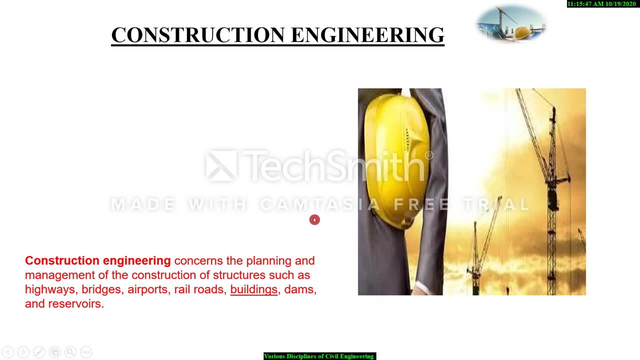 the ground and here in this picture a pile is inserted as the foundation. other important branch or the discipline of civil engineering is the construction engineering. so the structural engineer will design, will analyze and design a structure and the geotechnical engineer will focus on how it can be founded on. 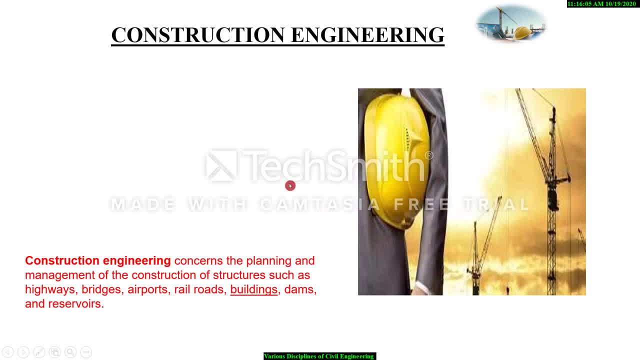 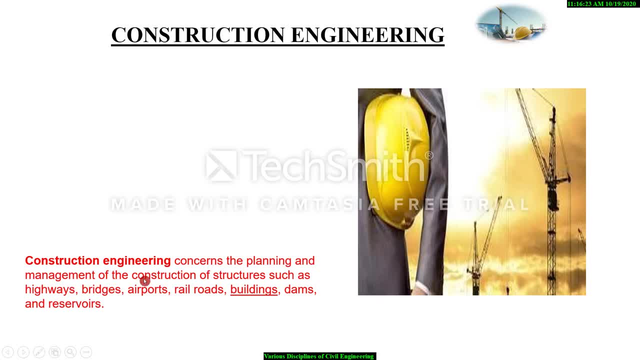 engineering concerns the planning and management of the construction of structures such as highways, bridges, airports, railroads, buildings, dams and reservoirs. anything which is design has to be executed by the construction engineer and that branch is called as construction engineering is involved in planning and planning. so he is involved in planning and 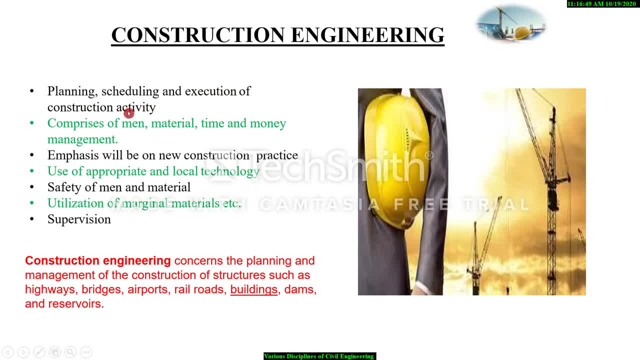 scheduling and the execution of the construction activity. he should manage or organize the main material, time and money should. emphasis should be there on the new construction practice for the faster construction and for the money savings and you should be well known about the appropriate and the local technology if it demands. should ensure the safety of the men and material. also. 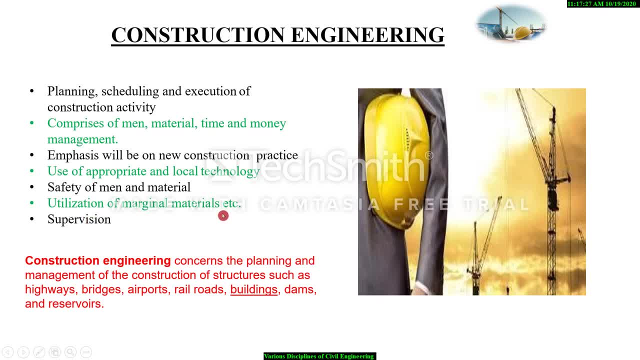 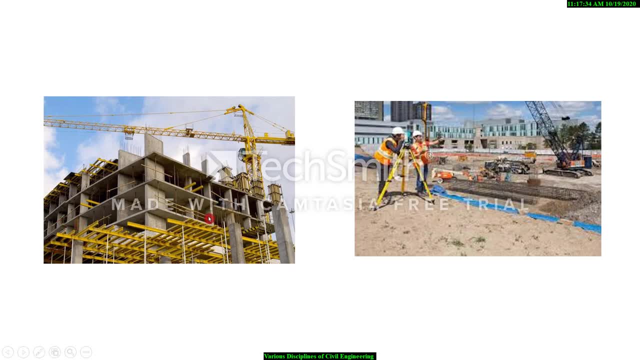 you should properly utilize the marginal materials and he should supervise all the box. so this figure shows a construction work by paper and paper, big, flat, and here you can see the is basically survey engineers which is doing in the land survey well before the construction. so the construction 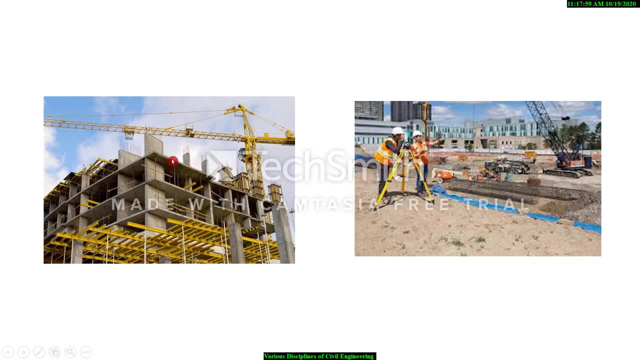 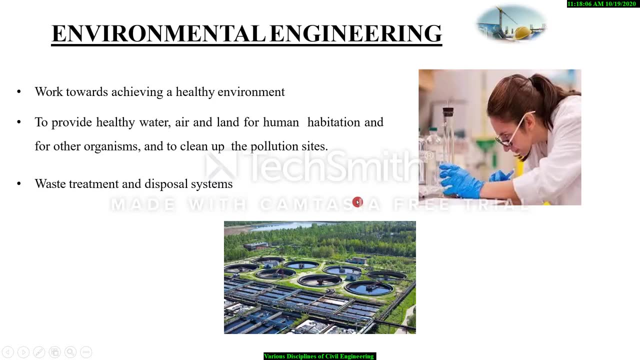 engineers should also make sure that every construction is going in proper way and in the proper alignment. the other important discipline of civil engineering is the environmental engineering. environmental engineers works to aids for achieving a healthy environment, so they are basically on the environmental part, providing a good living condition. 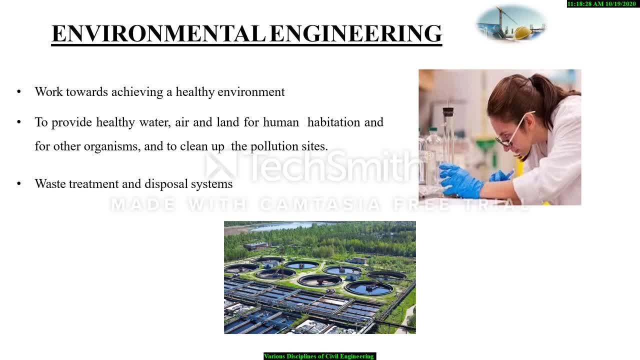 so they are. environmental engineers are in charge of providing the healthy water, air and land for the human habitation and for other organisms, and also to clean up the pollution sites. they should work and maintain the environment, and they should design the proper waste treatment technologies and waste disposal. 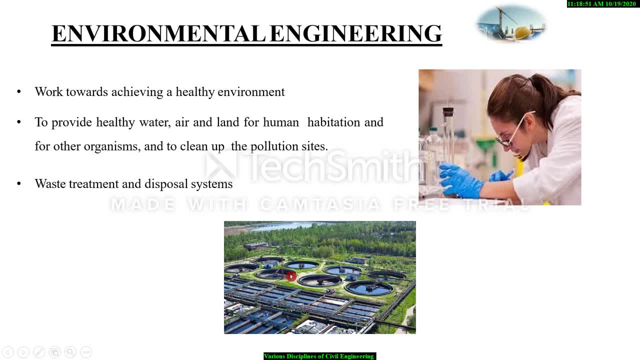 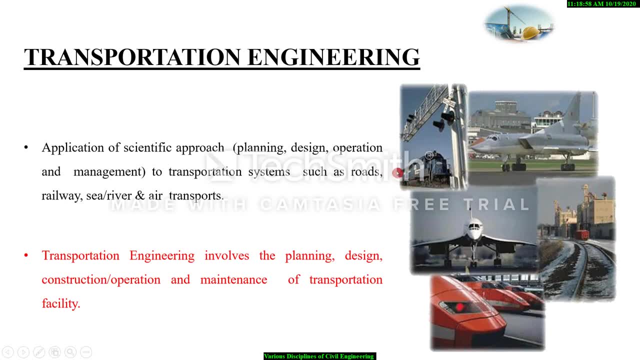 systems, some advanced, environmental, like the water treatment plants. the other important discipline of civil engineering is transportation engineering- this is very clear from the IT translation, but which will be having anything that roadway, airway, waterway, anything can come under the transportation engineer. so it's basically application of scientific approach: planning, designing, operation and 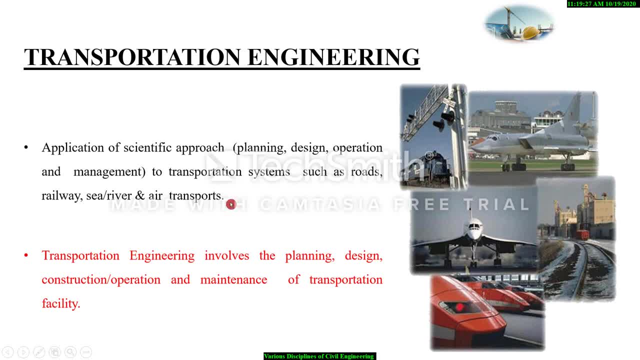 management to the transportation system, such as roads, railway, sea or river and air transport. such a definition, transportation engineering, involves the planning, design, construction or operation and maintenance of the transportation facility. so there was one behind making the roads or broadway or airports and, like for the railways, the slippers, tracks, everything. 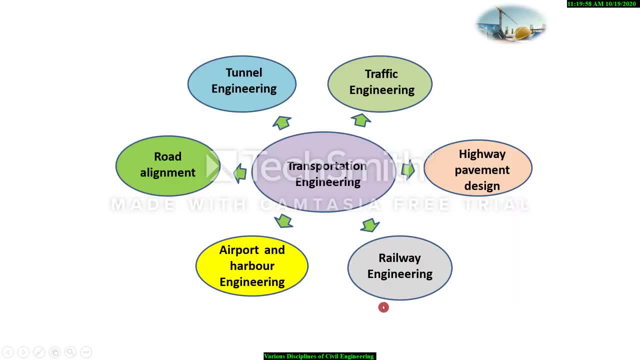 and there are some submissions for, even for the transportation engineering. they are like the tunnel engineering if the tunnel is used for the vehicle movement. so the there's a requirement of audio engineering engineer and the production engineer. so trial engineering is subdivision, traffic engineering, traffic management, the highway pavement design. 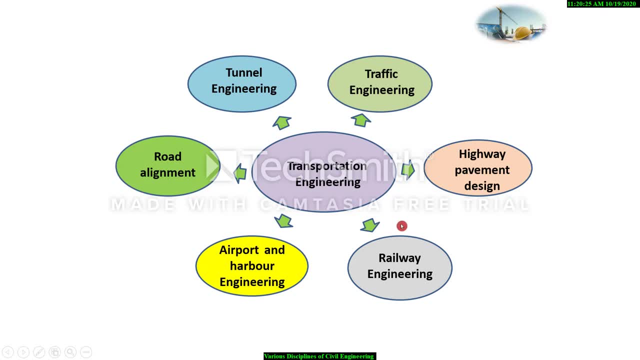 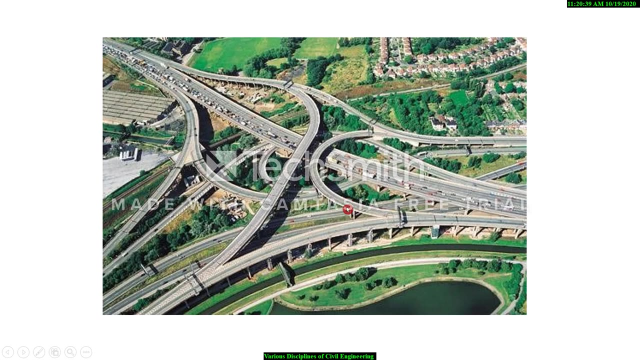 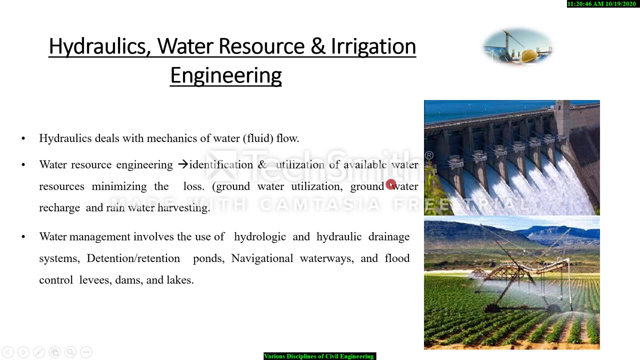 is also a specialized subject under the transportation engineering and we have the railway engineering, airport and harbour engineering, road alignment. this shows a very advanced rotary intersection or interchange for the of a traffic management. other important discipline is the hydraulics, water resource and irrigation engineering, so the hydraulics bird. it means that it. 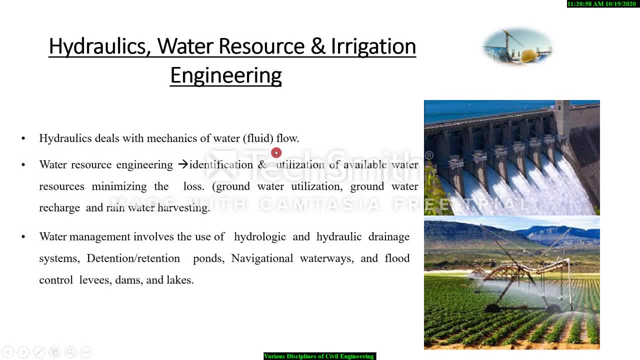 deals with the mechanics of water flow. the water resource engineering is about the identification and utilization of the available water resources by minimizing the flow of the water. this goes overを see in the laws, so we can use the groundwater and relay on the groundwater recharge and the rain harvesting for the efficient. 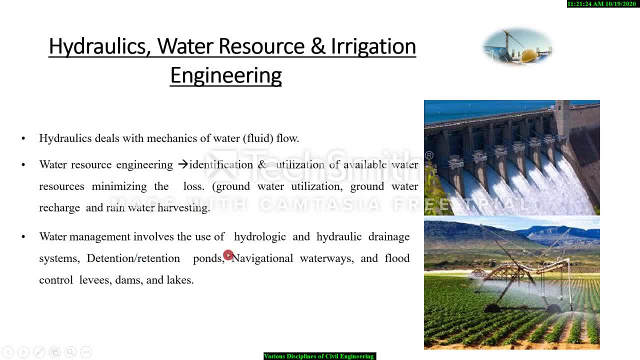 water management involves the use of hydraulics and hydraulic drainage systems, attention or attention ponds, navigational waterways and the flood control levees, dams. so these are some advanced thing which are used for the effective water management. So you can see, the making of dams and other canals requires some expertise from the hydraulics.